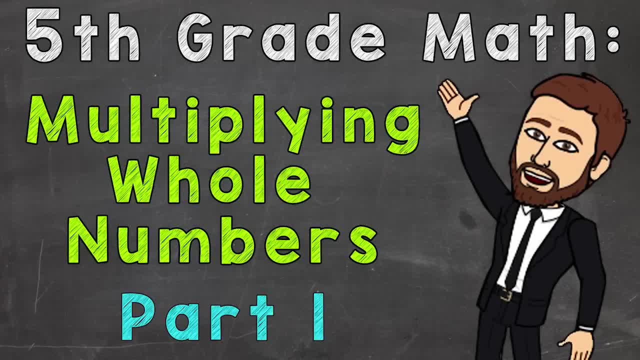 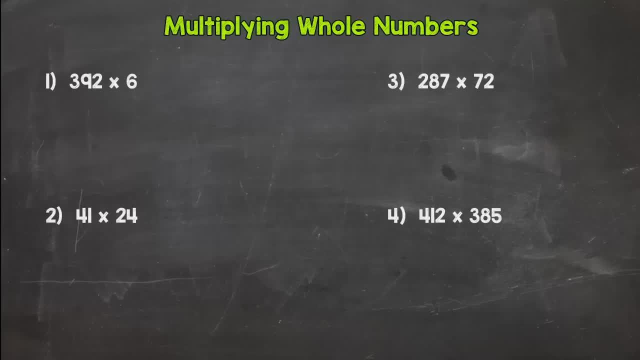 Welcome to 5th Grade Math with Mr J. In this video, we are going to be learning how to multiply whole numbers. Okay, and as you can see, we have four multiplication problems on the screen there. So what I suggest as we go through these. if I were you, I'd be writing these along with me. 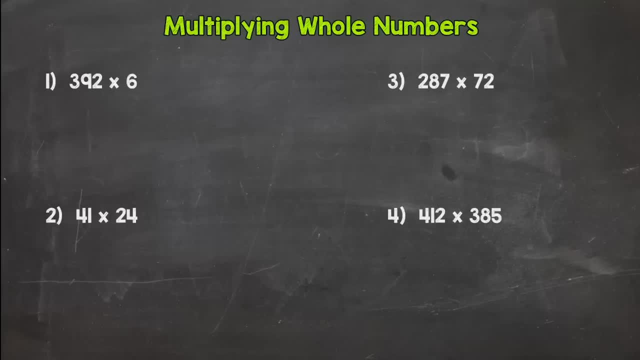 Even if you're not sure what you're doing, that will be helpful. writing these out with me on a piece of paper And we'll go through some examples here. Obviously, we have four, like I just talked about, and, as you can see, 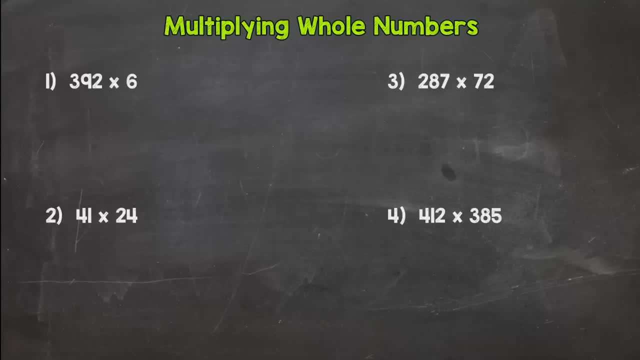 And after we do these four, we'll follow up with a mastery check where you can try some on your own. Okay, so if you know your math facts, your basic multiplication facts, these really aren't going to be too bad, Because as we go through the process of multiplying larger numbers, here it's nothing but just little facts combined together to give us our final answer. 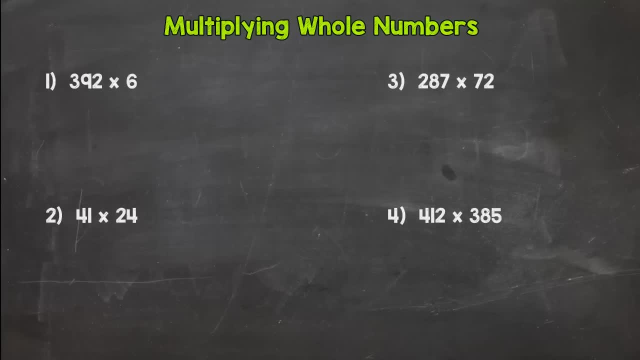 Okay, so we're going to go through this. We're going to hop into number one here and just go through our process. So we are going to line up our problem vertically, which means up and down, Okay, and there we go, 392 times 6.. 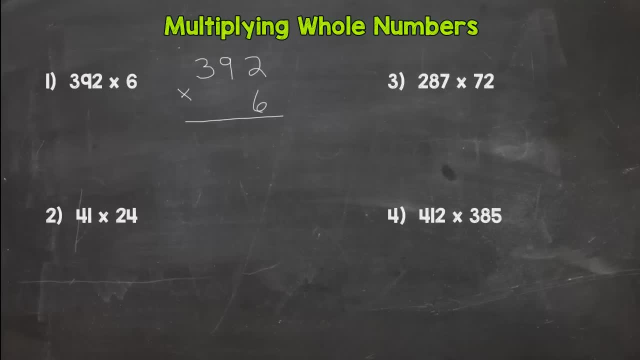 So the first thing we do, we take the 6 times 2,, which is 12.. Then we take the 6 to the 9.. 6 times 9 is 54.. 4 plus that 1 is 55.. 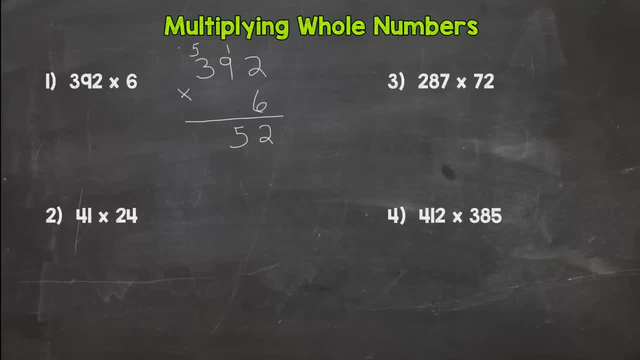 6 times 3 is 18.. Plus that 5 is 23.. Put our comma in there: 2,352.. Okay, Number 2.. We have a 2 by 2, which is going to be a little different. 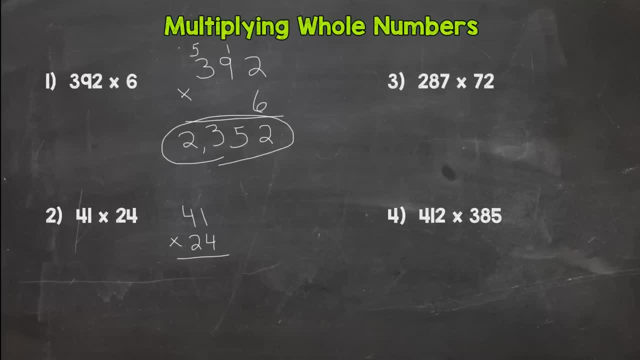 Hopefully, going into 5th grade You have a 3 by 1 down right Or a 2 by 1.. You know that process. So in 5th grade this 2 by 2 here might be a little new to you. 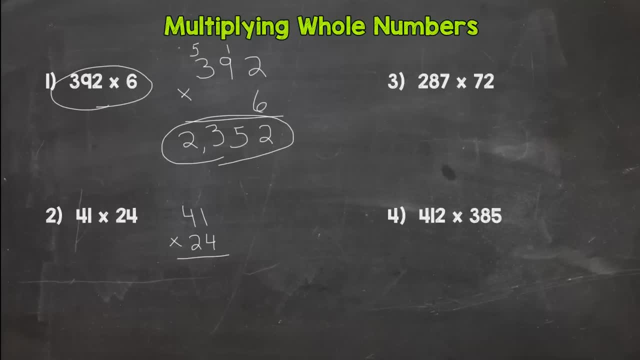 Okay, and that's fine. We start the problem off the same way. we did this top one. here We take the 4 to the 1 and the 4 to the 4.. So we would start by going 4 times 1 is 4.. 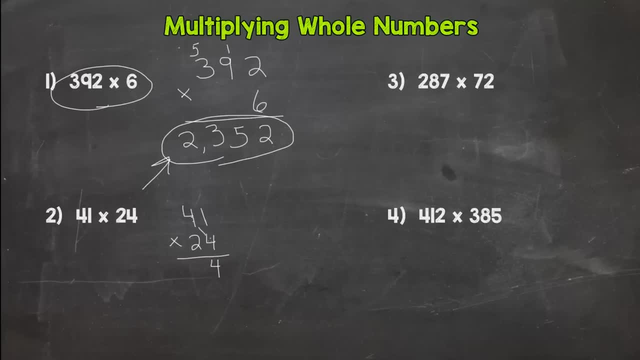 And 4 times 4, take it up here- is 16.. So we get 164.. That is not our final answer, though. Okay, We are done with this 4, so we can cross it off. We're done with the 4.. 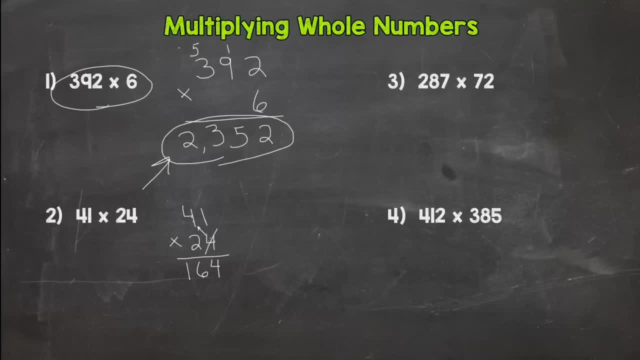 Now this next step is very important. If you forget this, you are not going to get the correct answer. Okay, So we're going to do this, We're going to do this. What is the value of this 2?? Hopefully you are thinking to yourself- 20.. 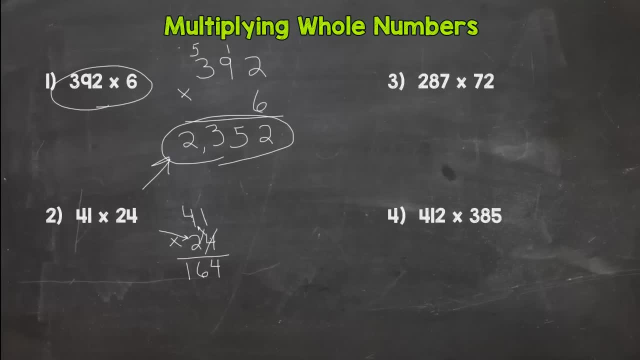 We are multiplying a 20 times this 1 and a 20 times this 4.. So, in order to do that, we are going to put a 0 here, a placeholder 0. Because this 2 is worth 20.. And then we take the 2 to the 1.. 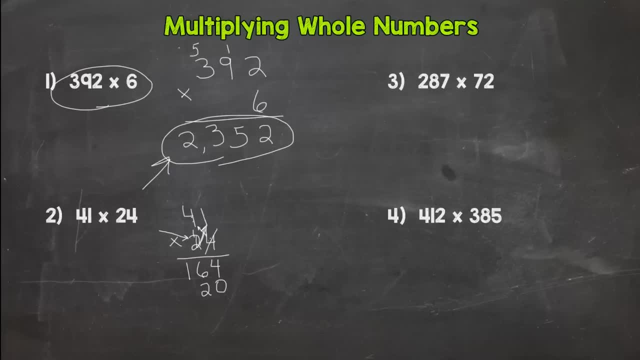 2 times 1 is 2., And then the 2 to the 4.. 2 times 4 is 8., And then we add these two numbers together to give us our product. And the product is an answer to a multiplication problem. 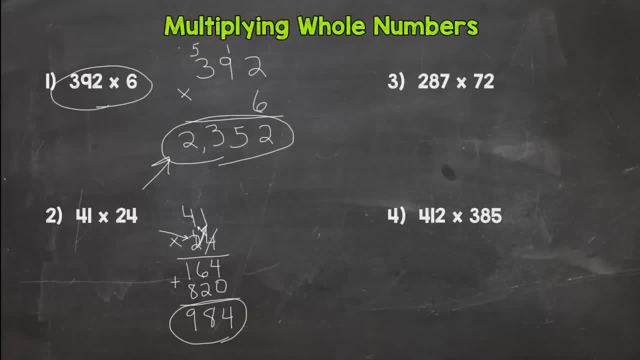 So our answer is 984.. Okay, This is our product, Our answer And what we added here together to get our product. these are called our partial products. Think Part of the product. They are part of our answer. Our partial products give us our product. 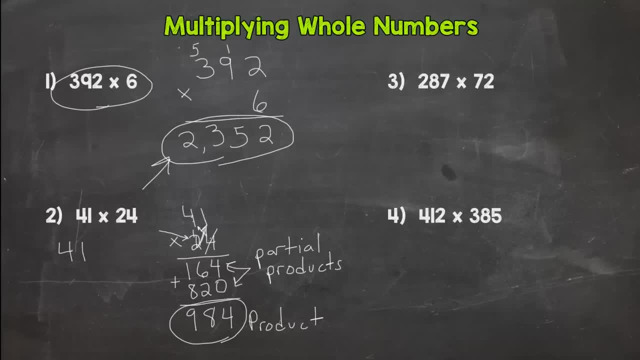 Okay, I'm going to show you what not to do over here to the left You do not do. 4 times 1 is 4.. And then 2 times 4 is 8.. Answer 84.. This would be incorrect. 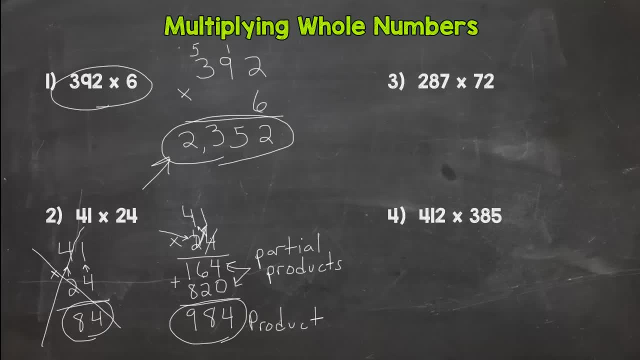 Okay, Let's try number 3. here We're going to step it up a notch. We have a 3 by 2.. So we start by taking the 2 to the 7,, the 8, and the 2.. 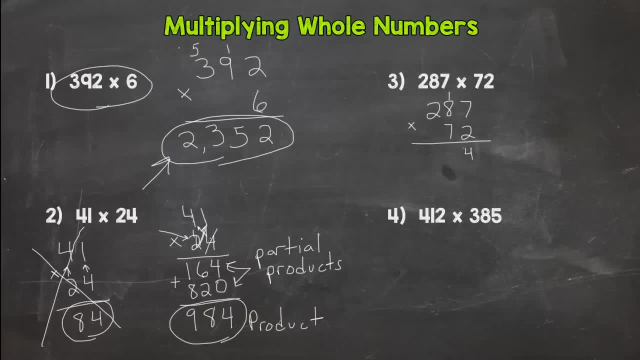 So 2 times 7 is 14.. 2 times 8 is 16.. Plus that 1 is 17.. 2 times 2 is 4.. Plus that 1 is a 5.. We are done with this 2.. 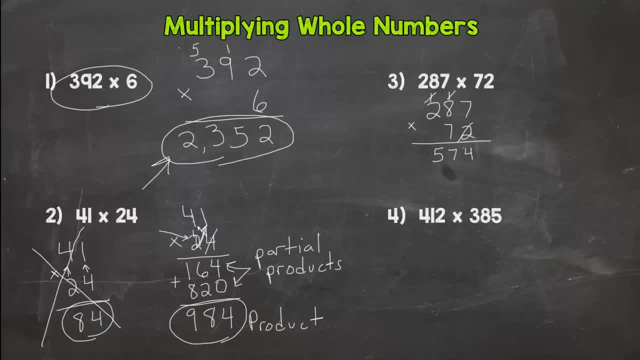 And we are done with our regrouped 1s up top. So I like crossing it off so I don't get confused with things. Now this 7 is worth 70.. So we are going to put a placeholder 0 there, making that 7 worth 70. 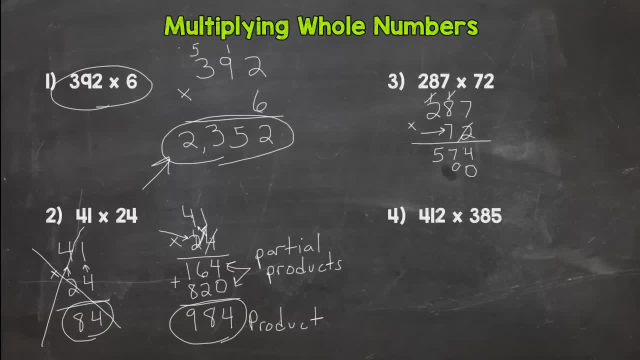 So we take the 7 to everything now: 7 times 7 is 49.. So I have a little 4 up here. That's why I crossed off the 1, so I don't get confused here. 7 times 8 is 56.. 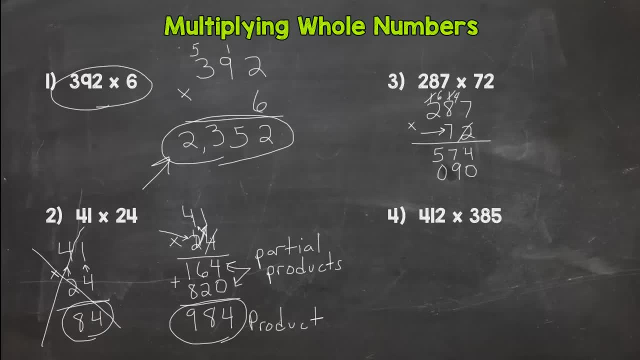 Plus the 4 is 7.. Plus the 4 is 60. Regroup my 6. 7 times 2 is 14.. Plus that 6 is 20.. So there we go. Those are our partial products. Make sure I'm nice and neat and I have everything lined up so I know what I'm adding. 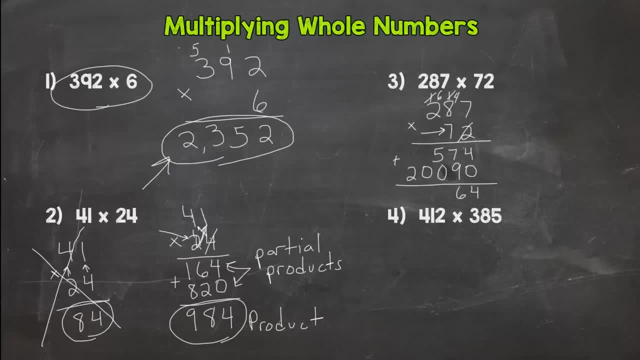 The 4 plus 0 is 4.. 7 plus 9 is 16.. 1 plus 5 is 6.. We have a 0 here And a 2. So our final answer would be 20,664.. 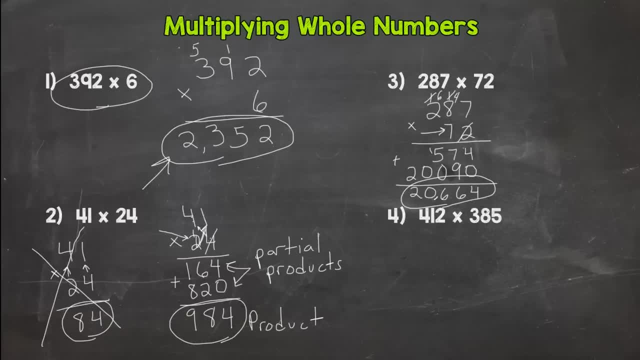 That would be our product. Okay. Next we have a 3 by 3.. We're going to need a little more room here. 412 times 385.. So let's start off by taking the 5 to everything. 5 times 2 is 10.. 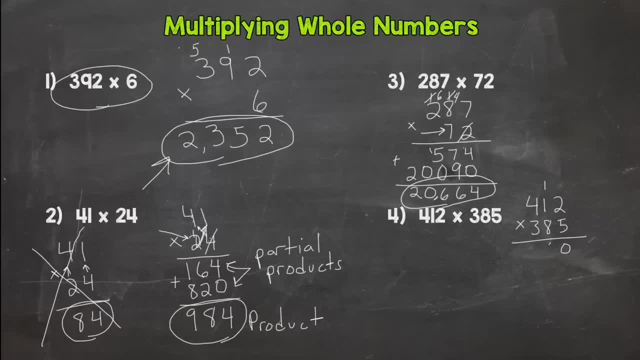 5 times 1 is 5.. Plus 1 is 6.. 5 times 4 is 20.. So we're done with the 5.. Done with that 1 up there. This 8 is worth 80. So we put a 0 there to represent that. 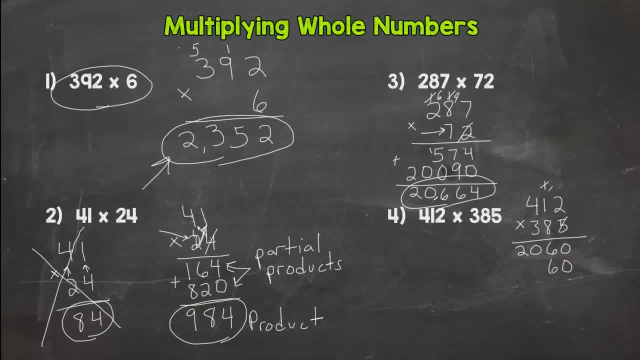 8 times 2 is 16.. 8 times 1 is 8.. Plus 1 is 9.. 8 times 4 is 32.. We're done with the 8.. In this problem, we're going to have 3 partial products added together. 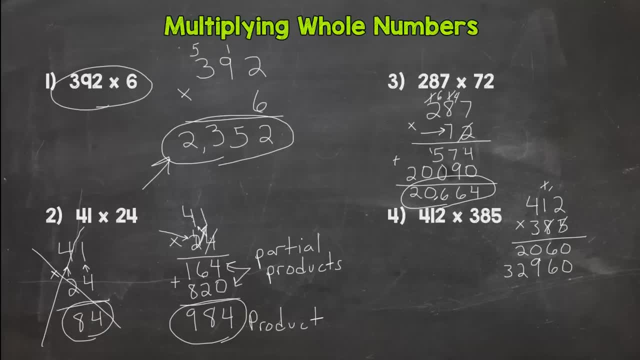 Because we have a 3 here: 300.. The value of that 3 is 300.. So we need 2 placeholder 0s if we go over to the hundreds place, Because that is worth 300.. 3 times 2 is 6.. 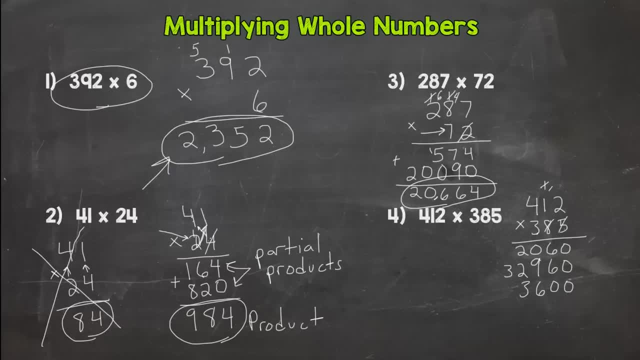 3 times 1 is 3. And 3 times 4 is 12.. And 3 times 4 is 12.. We have 3 partial products there. Because we have 3 digits: 385.. Okay, we took the 5.. 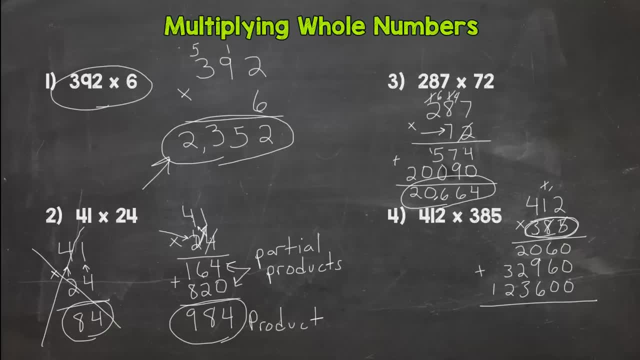 The 80. And the 300.. To each of the digits above in 412.. So let's add these together to give us our final product: 12., 16., 8., 5. And 1., So 158,620.. 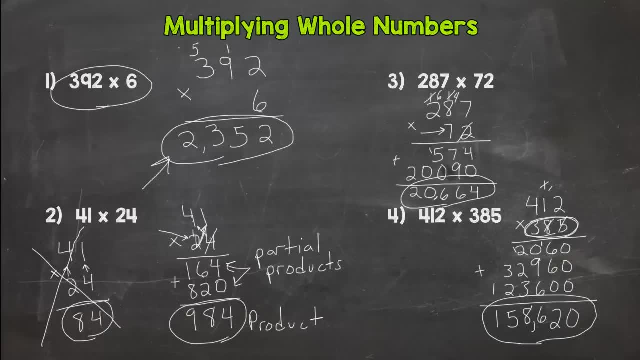 Okay, So those are 4 different types of problems there. We had a 3 by 1., A 2 by 2., A 3 by 2. And a 3 by 3.. Okay, so here's what we're going to do. 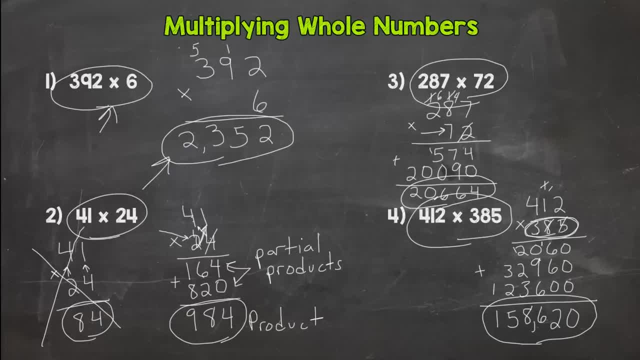 If you are confident in your ability to multiply whole numbers. I dropped the link to the mastery check below in the description. Go ahead over and try the mastery check to see if you have it down. If you want a few more practice problems to work out with me. 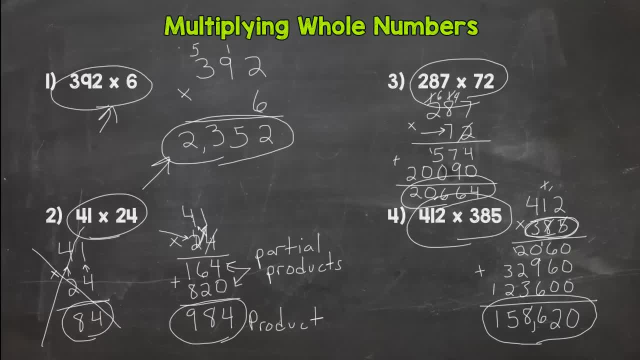 I will do a multiplying whole numbers, part 2. Where we will do 4 more problems just like these To have a little more practice, Okay, and then you'll try the mastery check. So I will see you over at part 2.. 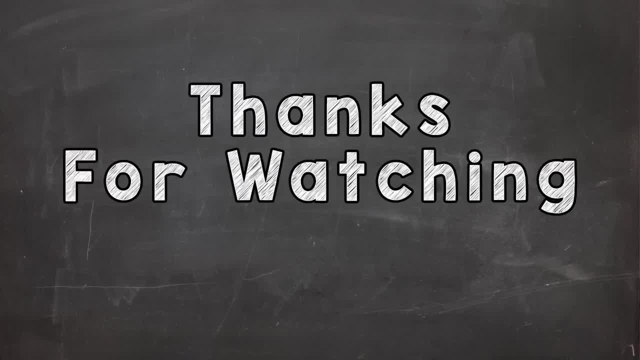 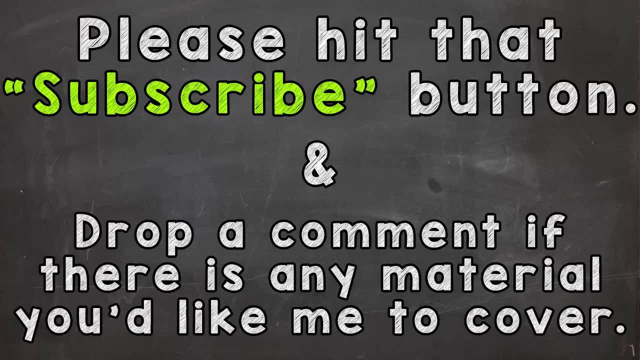 Or the mastery check. Thanks for watching. Please hit that subscribe button And let me know if there's any material you'd like me to cover Down in the comments. Until next time, Peace.